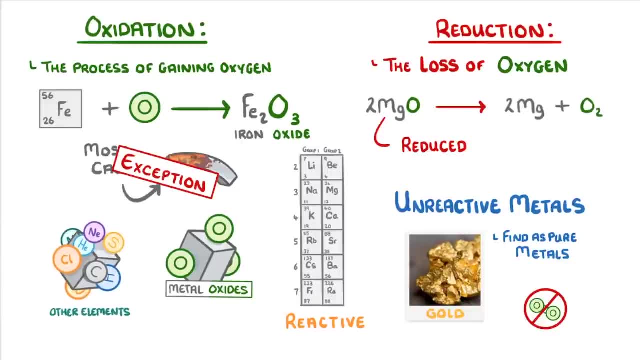 find metals bonded to other elements as well, but being bonded to oxygen is the most common and you need to know how we can remove this oxygen to get a pure metal. We saw at the beginning that reduction means the loss of oxygen, so essentially we're trying. 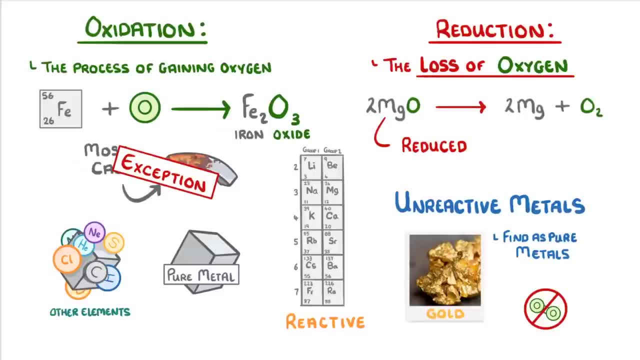 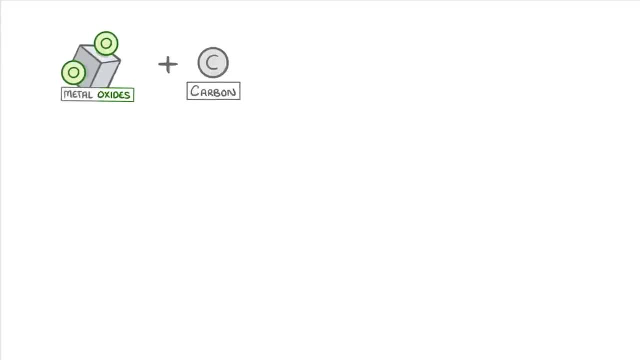 to reduce our metal oxides to get pure metals. The cheapest and easiest way to do this is to direct our metal oxides with carbon. The idea is that the carbon will basically take the oxygen from the metal to form carbon dioxide and leave behind a pure metal. 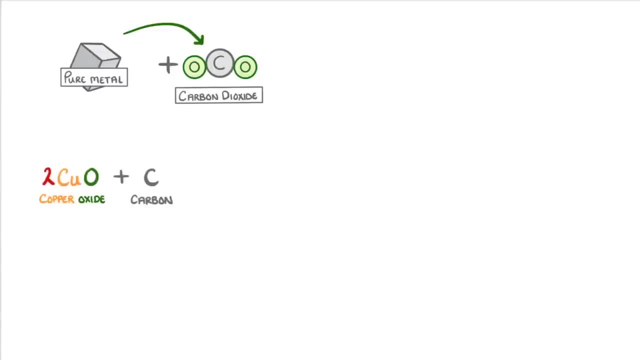 For example, a copper oxide plus carbon reacts to form copper plus carbon dioxide, So we would say that the copper was reduced because it lost oxygen and the carbon was oxidised because it gained oxygen. Unfortunately, though, we can't do this with all metals, only the ones that are less reactive. 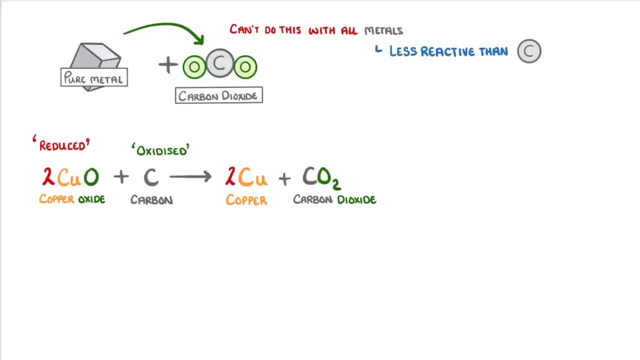 than carbon, And this is the reason why we place carbon in our reactivity series. We can see from this list that we can use carbon to form copper and carbon to form carbon dioxide. We can use the reduction with carbon technique to extract zinc, iron and copper from their 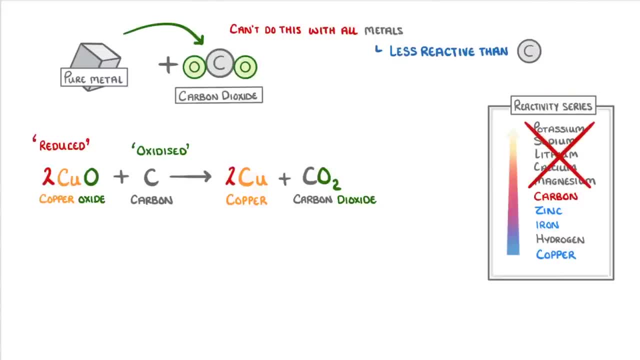 oxides, But we couldn't extract any of these more reactive metals. For these ones we'd have to use a process called electrolysis, which we'll cover in another video, but basically requires loads of energy and so is really expensive. 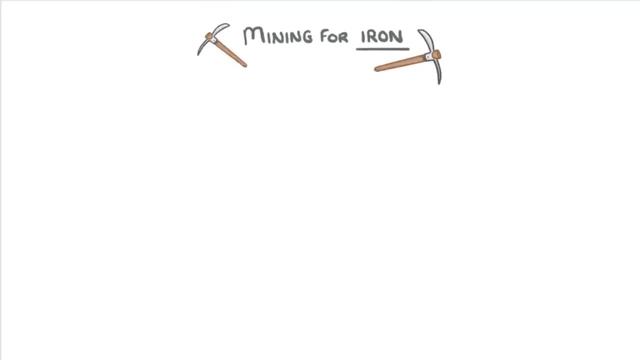 As a last example of using carbon, let's imagine that we were mining for iron. As we take the rock from the ground and separate it from the metal, we can see that the iron is less reactive than carbon. If we were to separate out the bits that contain iron, we'd find that we have lots of different. 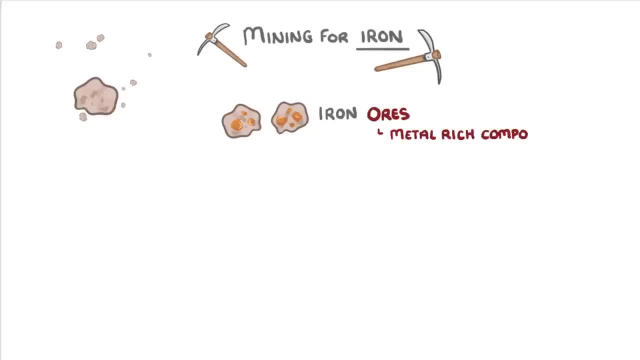 iron ores, with ores referring to metal-rich compounds that we can extract our metal from. The most common ore will be Fe2O3, which is a type of iron oxide. So to isolate the pure iron, we need to reduce this iron oxide to just iron. 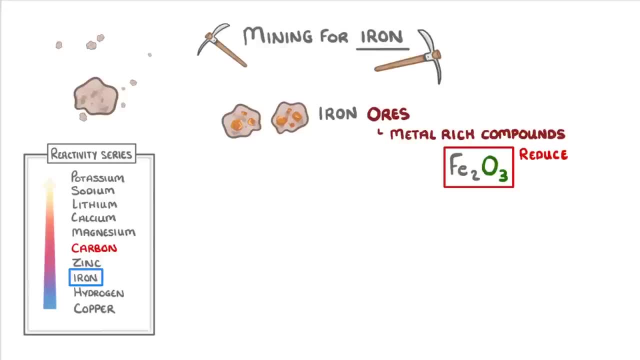 If we check our reactivity series, we can see that iron is less reactive than carbon, So we're able to do reduction with carbon and we can see that the iron oxide that we've with carbon, rather than having to do electrolysis like we would with these.